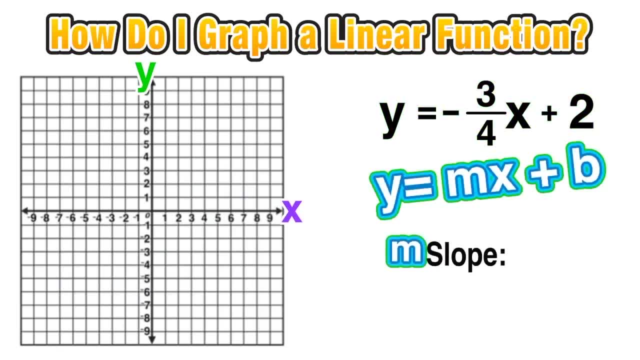 b form, That's slope intercept form, And when it's in this form it's actually pretty easy to graph. So we can see that our slope is going to be that negative 3 over 4.. Okay, and when we have a negative slope, we know that our line is going to be descending from left. 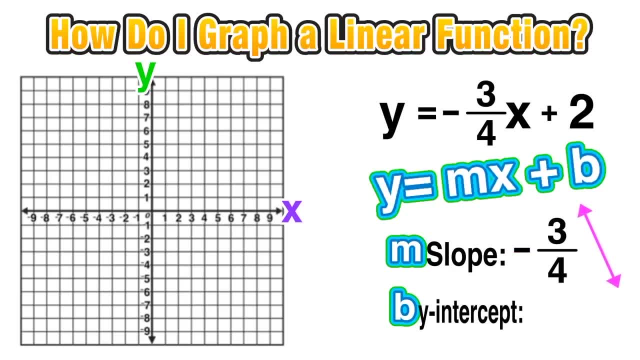 to right. So we should have somewhat of an idea of what our line is going to look like when we do graph it And the next thing that we see is that our y intercept, that b value, is at positive 2.. So we know that the graph is going to hit that y axis at positive 2.. So the first step, 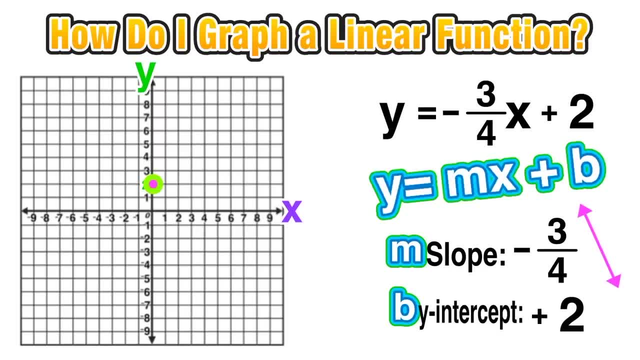 to graphing a linear function in slope intercept form is to plot that y intercept. In this case, I'm putting a point at positive 2 on the y axis And now we're ready to build that line from that point. Now that slope of negative 3 over 4, I'm going to take the negative sign. 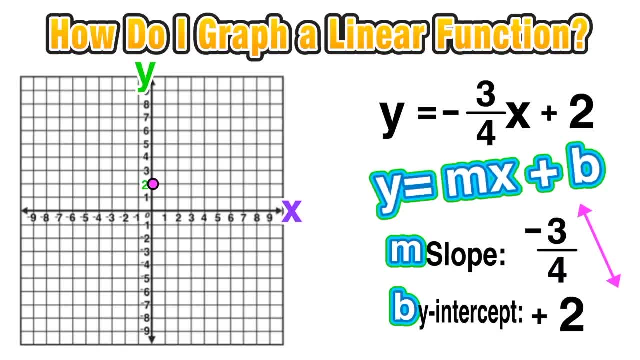 and push it up to the value in the numerator. Okay, so I put it with the 3 to make it a negative 3.. And if we think of slope in terms of rise over run, as in change in y over change in x, So when our rise is negative 3, think of that as rising down. We're going down 3 units. 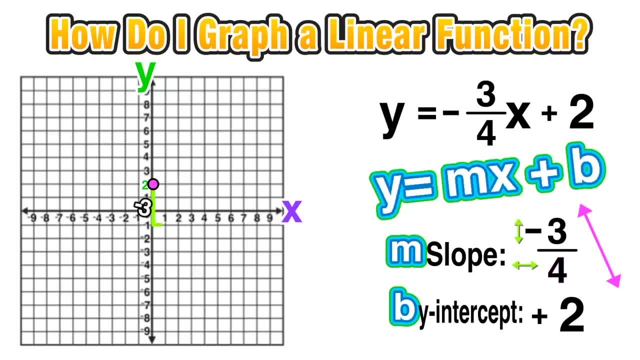 on the y axis And then our run, our change in x is a positive 4. So we move to the right 4 units and then we plot a new point, And we can continue to build off of each point, in this case our new point by repeating: 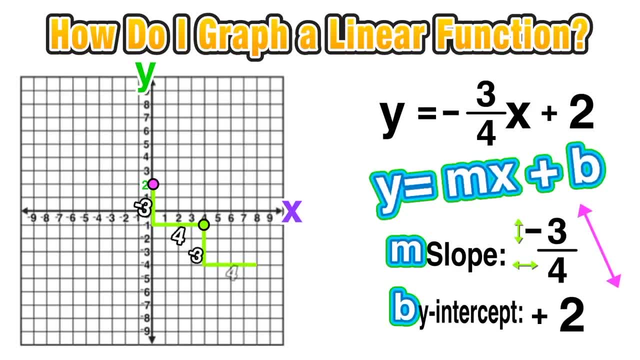 that slope. Again we rise down 3 units and then run to the right 4.. And again we plot another point. And if we are applying the slope correctly, we should see that we're building a pretty consistent staircase here. And if we want to plot some points on the 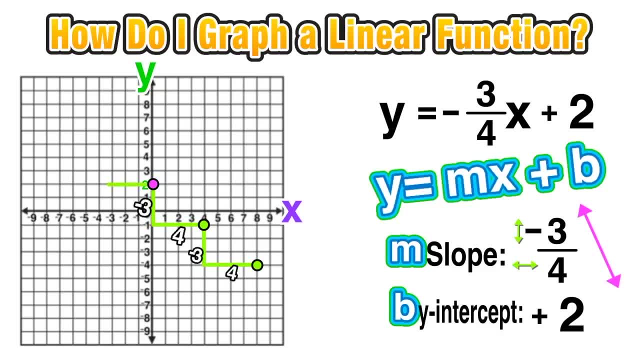 other side, on the left side of that y intercept that 2, we just repeat this process in reverse, In this case going to the left 4 units And then up 3 and plotting another point, And we should still see that our points are. 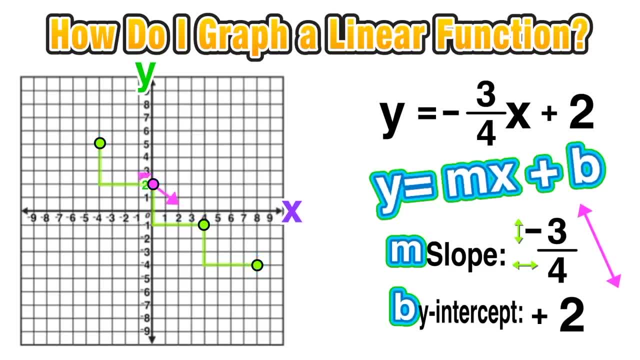 all aligned, Which means that we can construct a line that passes through all the points. And now we have successfully graphed our linear function: y equals negative 3 over 4x plus 2.. And just to reiterate again, the graph that we just constructed is the same thing. 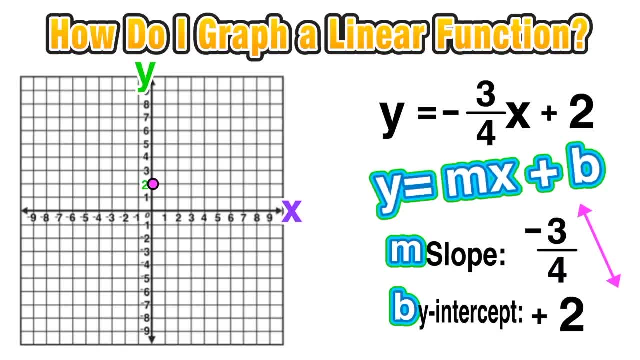 and push it up to the value in the numerator. Okay, so I put it with the 3 to make it a negative 3.. And if we think of slope in terms of rise over run, as in change in y over change in x, So when our rise is negative 3, think of that as rising down. We're going down 3 units. 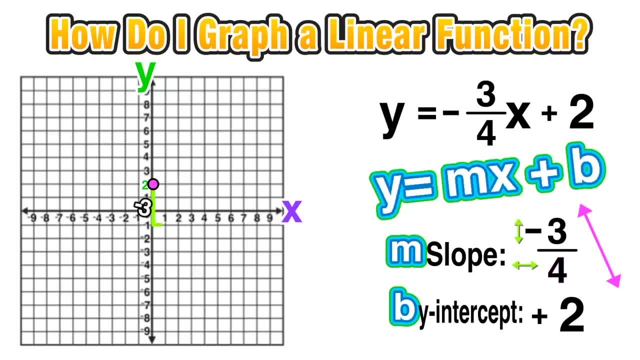 on the y axis And then our run, our change in x is a positive 4. So we move to the right 4 units and then we plot a new point, And we can continue to build off of each point, in this case our new point by repeating: 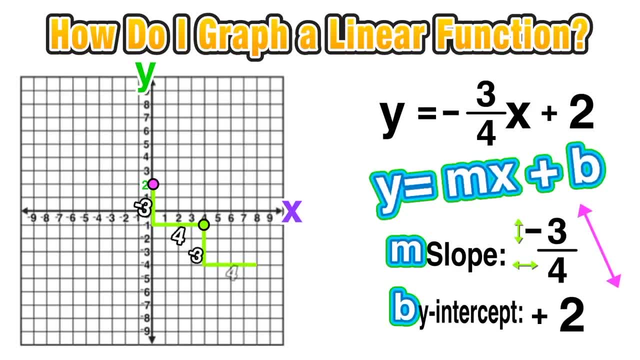 that slope. Again we rise down 3 units and then run to the right 4.. And again we plot another point. And if we are applying the slope correctly, we should see that we're building a pretty consistent staircase here. And if we want to plot some points on the 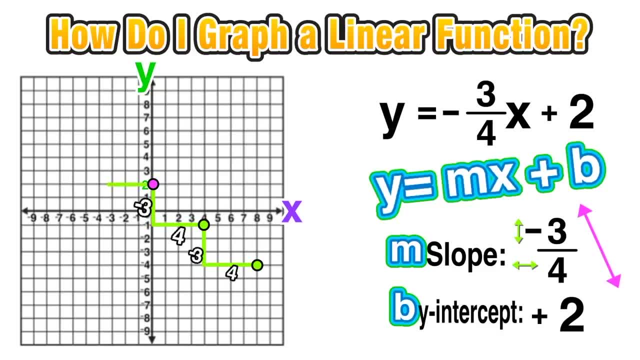 other side, on the left side of that y intercept that 2, we just repeat this process in reverse, In this case going to the left 4 units And then up 3 and plotting another point, And we should still see that our points are. 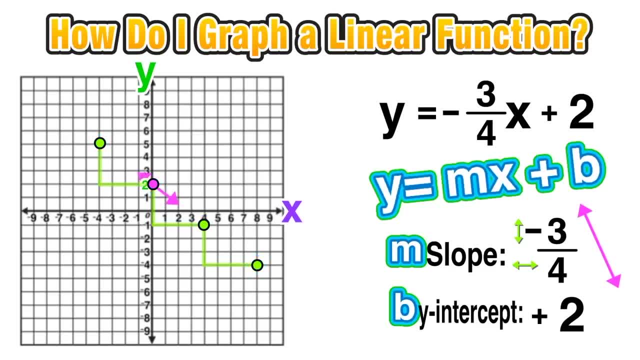 all aligned, Which means that we can construct a line that passes through all the points. And now we have successfully graphed our linear function. y equals negative 3 over 4x plus 2.. And just to reiterate again, the graph that we just constructed is the same thing as the. 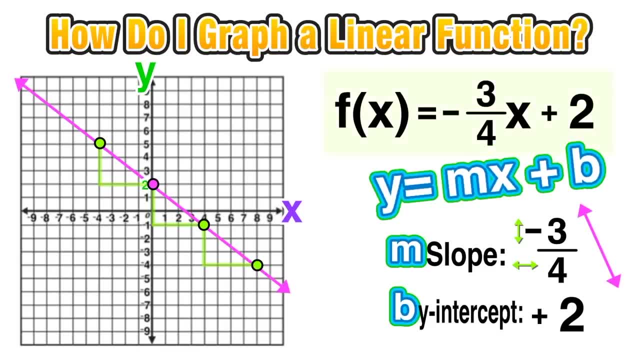 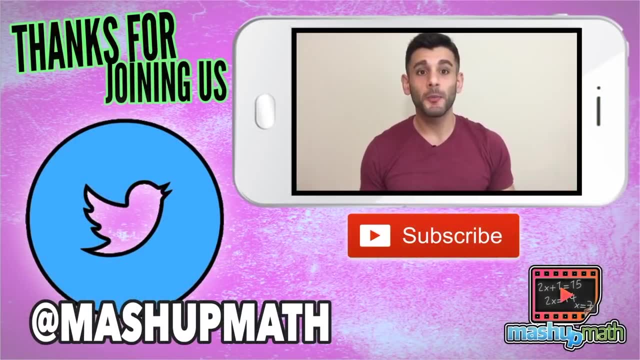 function f of x equals negative 3 over 4x plus 2.. So remember that y equals and f of mean the same thing, and that's all there is to it when it comes to graphing a linear function, and we'll catch you guys next time, haha, cool, all right, so that's it for that lesson hope you found. 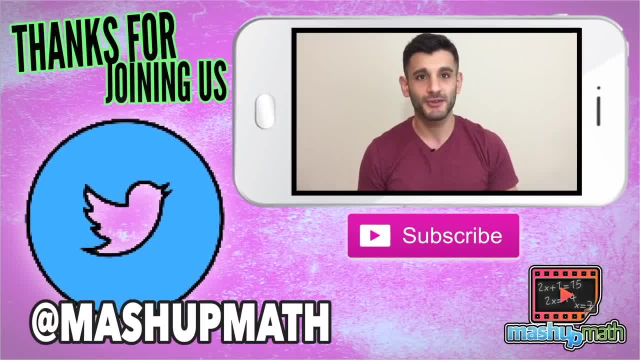 it helpful and, if you did, please click that link below and subscribe to our youtube channel. we add new lessons every week. we don't want you to miss out, and also, if you have any questions or concerns, feel free to comment down in the comment section below. we respond to every single. 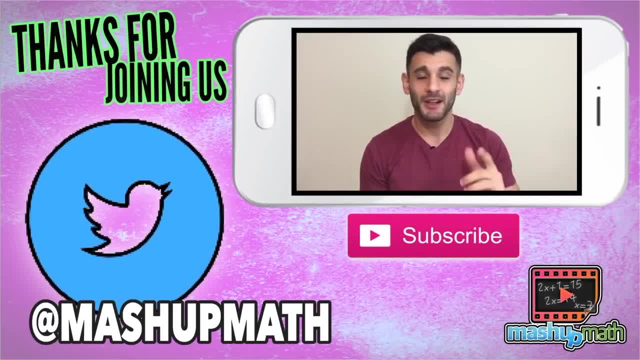 comment. i promise you will respond, even the mean ones, okay, but let's just try to keep it nice. those ones are always a lot more fun to read and we'll catch you guys next time, see ya.